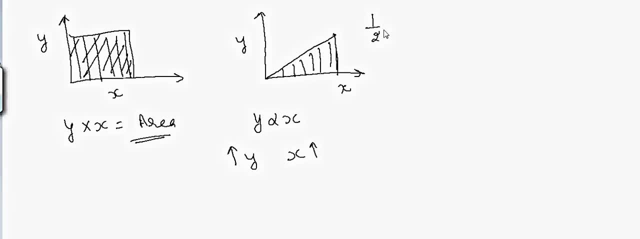 because this is a triangle, i know is half into y, into x, but yeah, you know it, but you can. you could also have a different shape. instead of being a straight line, it could have been like this, and then i would have to ask you how to calculate the area under this. so, not exactly like this. it. 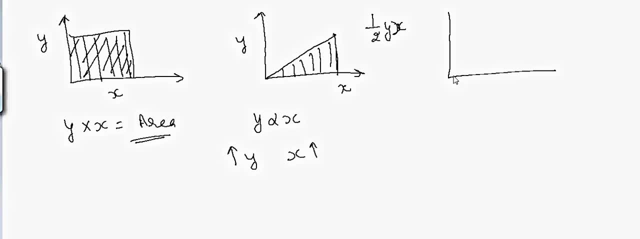 cannot be this, but let's, let's say it's like like this: so if you need to calculate this area, then how will you do it? so? so i'm giving, i'm using this uh triangle as an example, because that is more easier to describe, and then you can always go to the difficult ones. but now see, so how will? 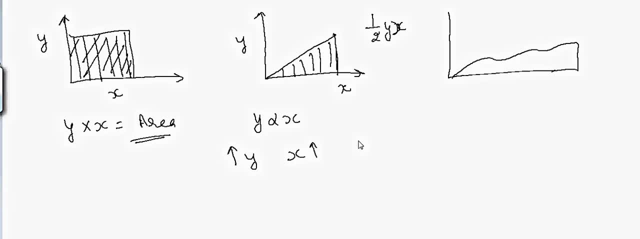 you define it. so now, y is proportional to x, and so suppose y is equal to a, a, a a to x. so what is your a? a is your constant. so it could be one or it could be anything else. so now we have to calculate the area. so you say: my area is equal to y into x. so that is true, right? 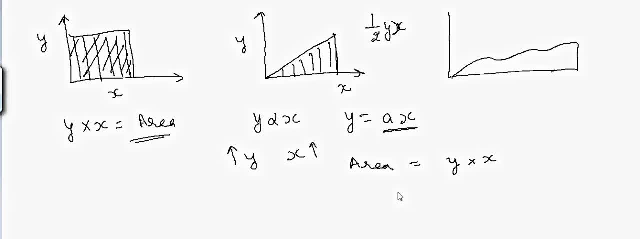 however, the y is changing. so y is equal to f of x. y, what is y is equal to f of x, the f of x, f of x means that y is the function of x. so you can see here: y is the function of x. so as you change uh x, your y also changes. so so what we have to do is we have to say: 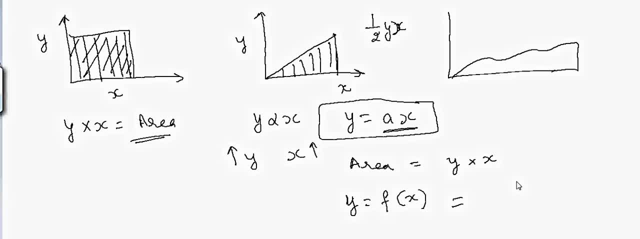 uh, that y um. so we will say a into x, into x, right, but now this x is not, cannot be. i'm not talking about this, is not x here. so we are talking about the small quantity, right. so so let's take, let's draw this again. 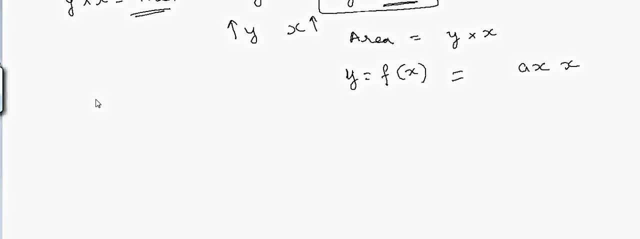 so what i can do is and draw this again and look at this way. now suppose i take a very, very small area like this and if i look at this area and i look at this part, so look at this part, so i can assume that this, in this area, the y is equal to y into x. so this is equal to y into x. so that is true. 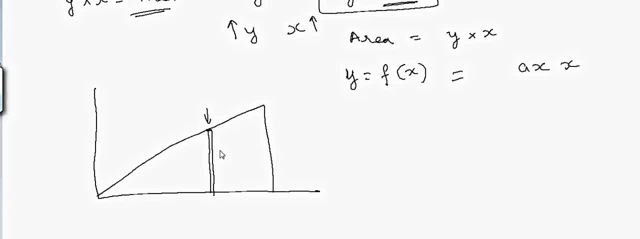 if i can forget this, and this is equal to oops. let me draw a smaller area. i can't think of what that is, but we can see that the y is like, so y is not changing. so i can say that y is constant in there because i've taken a very, very small area. so this area has to be very, very small, so half. 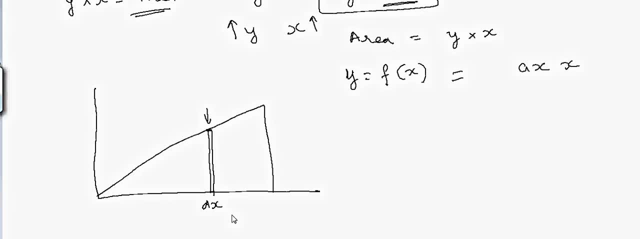 small. it should be almost close to zero. so we call this as so what? we call this as dx. so, and this is equal to y, so this is the y. so so, at of this strip, how do we calculate? we calculate it by y into dx, right, and then, similarly, we calculate: 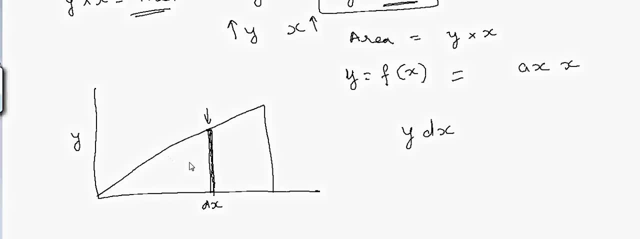 this strips. so we change the strip again now we take this area and we calculate this and then we add all the strips together to get to the answer. so to get to the area of this region, right? so what we do is we say add y, dx and change x from 0 to x. so this is your x. 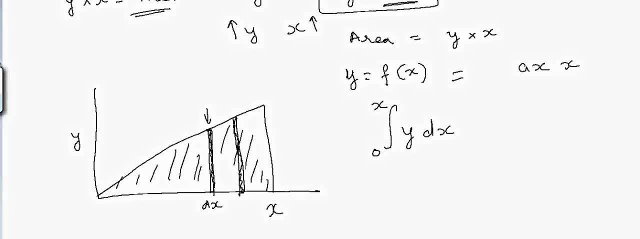 or we can, you can call it a capital x just for. so you need to define something, so let's, so let's call it capital x. this thing, right. so now, as you know that y is equal to a time x, so we can say y is equal to a x dx. 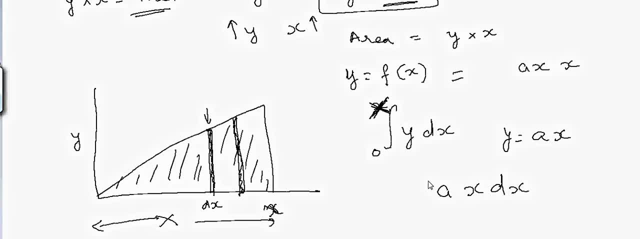 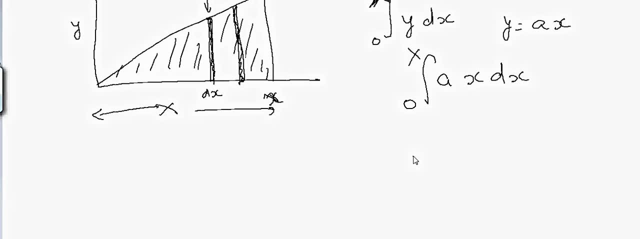 and then 0 to x, and now, if you define this one, then it will be equal to a into x square by 2. so this is your. now i'm using the standard formula for calculus, but so there is a way to uh to define this. but so you have to um. first you need to understand the 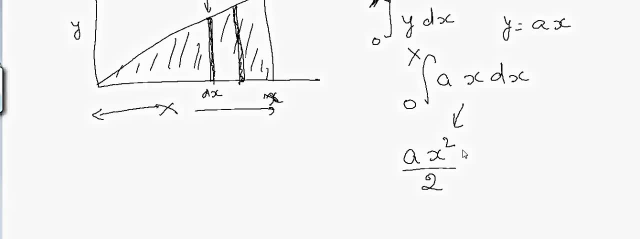 basic principles of calculus and then you can always remember these formulas. so if you do the simplification, it will be a x squared by 2, and then we'll say 0 to x. and if you do 0 to x, when you put 0 here it will become 0, and if you put x case, it will be a x squared by 2.. 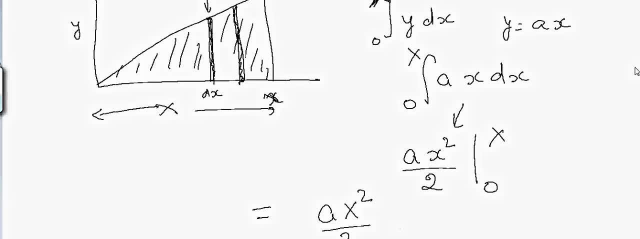 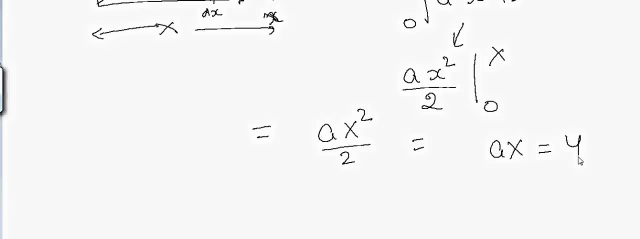 and as you know that, what is 2 or what is uh, a into x, a into x is equal to y, so you can say it's a, it's y, x right by 2.. so that is what you have. you already know this because it's the area of. 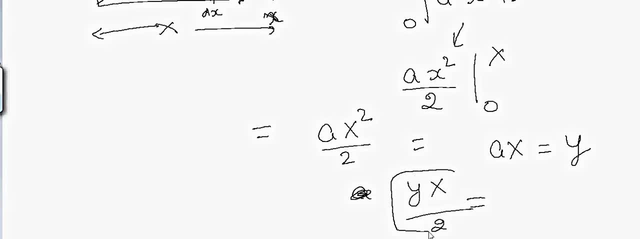 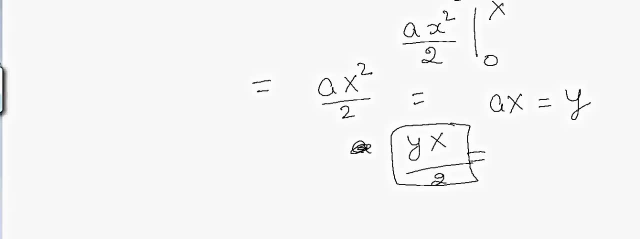 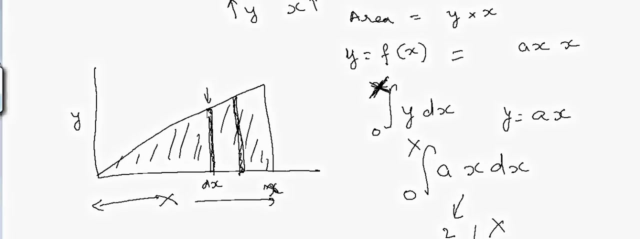 the triangle. but this is how you do. uh, go from calculus now. so this is what is the use of the calculus? so this is how you can define calculus. so you define each strip, you assume in that case, strip, small step, the y is not changing. and then, uh, you define everything in term of x, you integrate it. 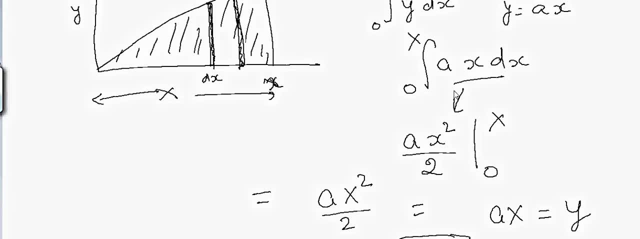 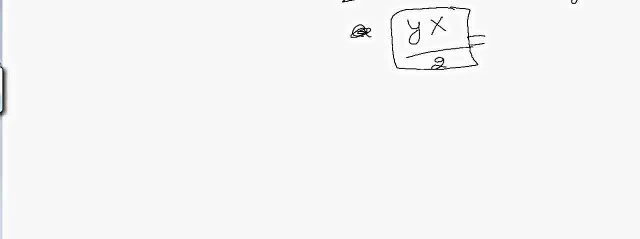 and then you can calculate the area. so similarly, like suppose um, um, when you have to calculate the velocity, uh, so this is your velocity, this is your time and the car is accelerating and it reaches a particular velocity, then we'll say how much distance it has traveled during this time. so 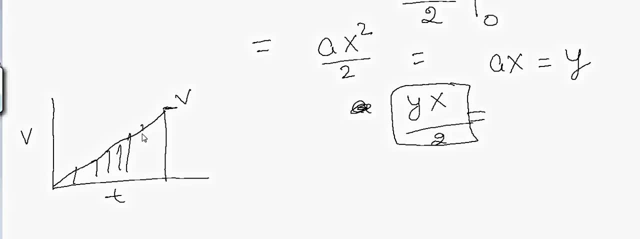 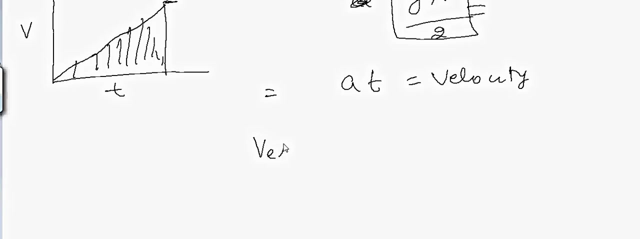 we'll. what we do is we say: acceleration into time is equal to velocity, right, so? so what we say is: velocity into time is equal to distance. however, velocity is changing with time, so we'll say: velocity is equal to function of time. so um. so we'll say um. 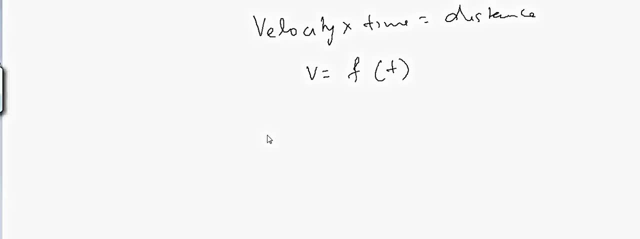 below: suppose velocity is equal to uh a time t, then uh, no, not a. let's define something else like: suppose b time t. so then in this case we'll be having um b time t into dt, dt by dt, because we are taking a small strip in this and then we are adding all the number of when t is equal to 0 to t. 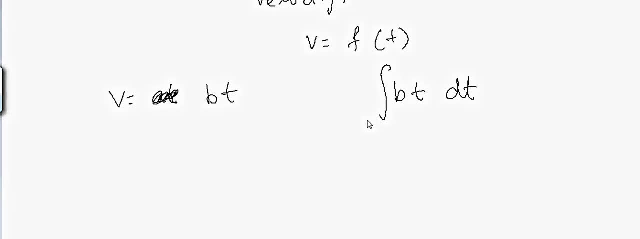 and that will be equal to b, t squared by 2, and you might have heard of it as so b, um, your, your b is nothing but a here. so b is um, because v is equal to b into t and uh. so if you, if you look at this, this is equal to uh, v divided by t, or is equal to a. so this is your acceleration.